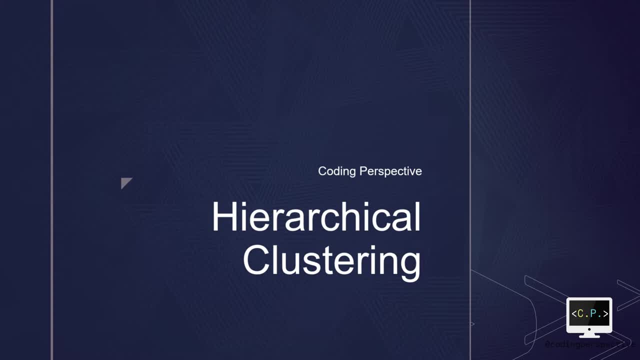 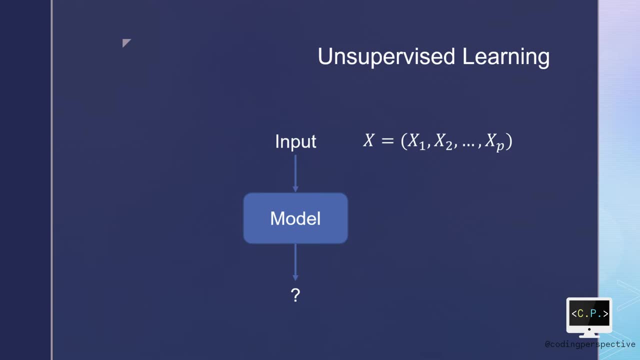 work in practice. You can see those videos using the link above. Let us start. As you remember, we have two types of learning algorithm: classes: supervised and unsupervised learning. So far we have seen supervised algorithms. Now we move on to the other type. 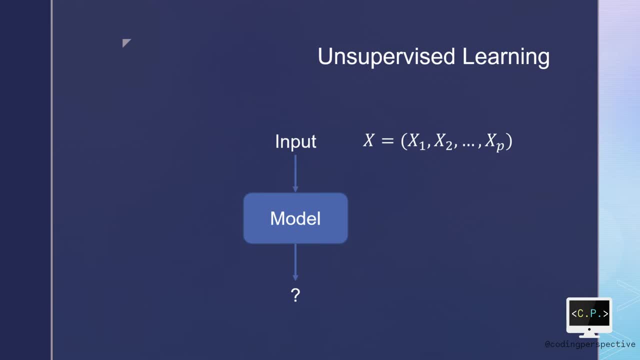 of learning tasks. that falls in the unsupervised learning class. This time we again have our data points, however without y-values, So there is no associated y-values in our data. We also have a reason for doing so, because a lived data model often prioritizes data. 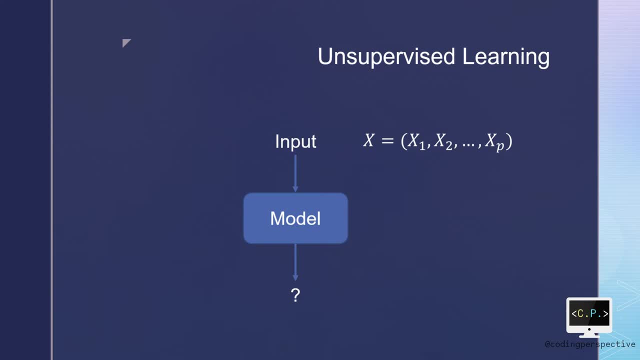 besides, due to the value of real values, We did choose our graph model and there was a working blind. This is referred to as unsupervised, because we do not have a response variable that can supervise our analysis. What do we do is that we seek to understand the relationships. 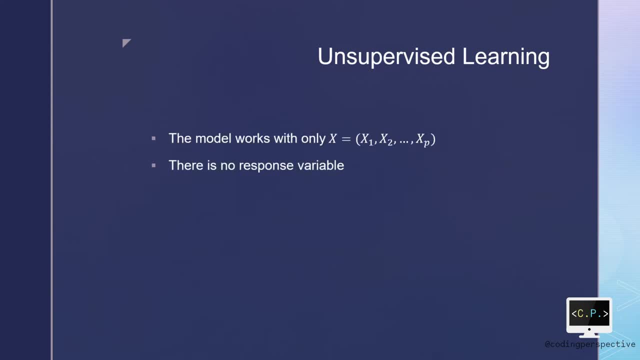 between the variables or between the observations. As said in the previous slide, there exist only x-values without their response variables With unsupervised statistical learning. there are inputs but no supervising output. Nevertheless, we can learn relationships and structure from such data. In general, we can cluster observations on the basis of the features. 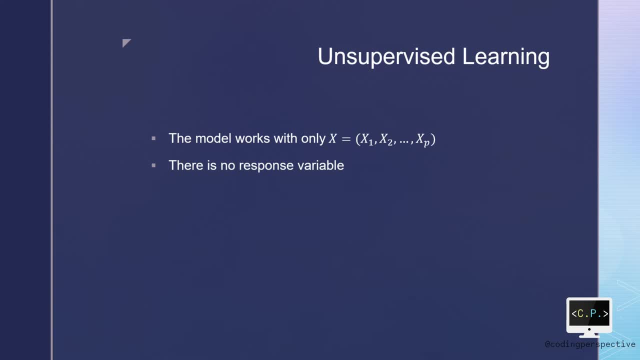 in order to identify subgroups among the observations, Or we can cluster features on the basis of the observations in order to discover subgroups among the features. Examples include customer segmentation, which can be used to identify subgroups among the features. A cluster image is a clustering task. Suppose that you are a manager of a store. 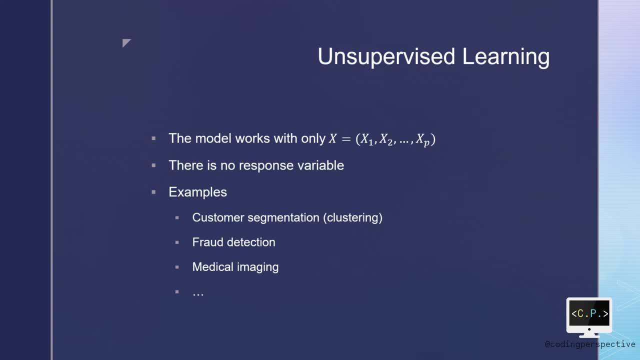 and you want to know your customers better than ever. How you could do this? Of course, it is not possible to focus on each individual. What you can do is that you can group individuals by looking their similarities. This operation is called clustering, Fraud detection, and some of the 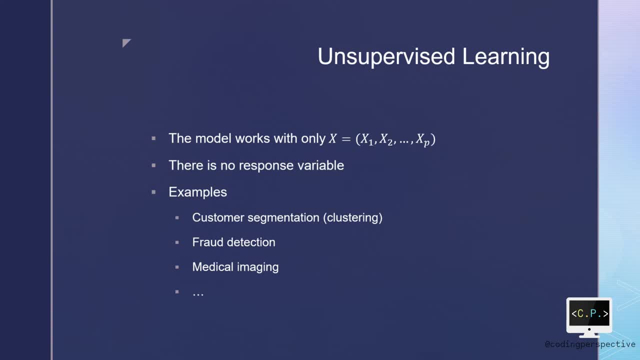 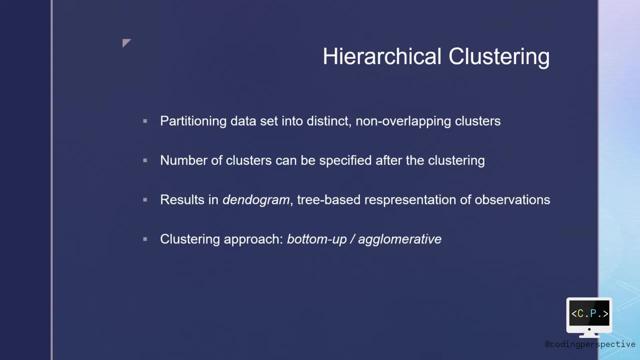 medical imaging can also be given as examples of this kind of learning tasks. Hierarchical clustering is a simple and elegant approach for partitioning a dataset into distinct, non-overlapping clusters, Comparing to k-means clustering. hierarchical clustering does not require to commit a particular choice of k, Thus number of clusters can be specified. 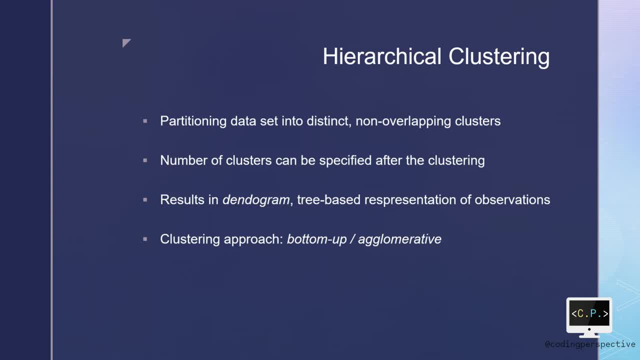 after performing the cluster incorporation. Hierarchical clustering has an advantage over k-means clustering which it results in an attractive tree-based representation of the observations, which is called a dendogram. There is a common approach to construct a dendogram which is bottom-up or agglomerative. This is the most common type of hierarchical. 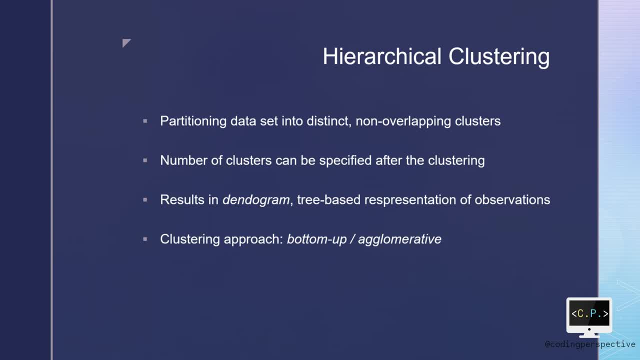 clustering and it refers to the fact that a dendogram is built starting from the leaves and combining clusters up to the trunk. We will see an example of a dendogram in the following minutes. The term hierarchical refers to the fact that clusters of height obtained by cutting the dendogram at a given height are necessarily nested within. 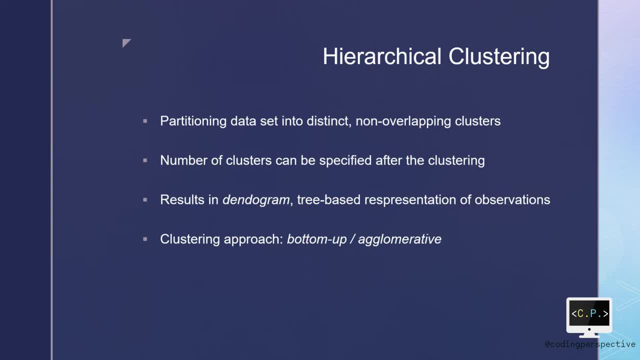 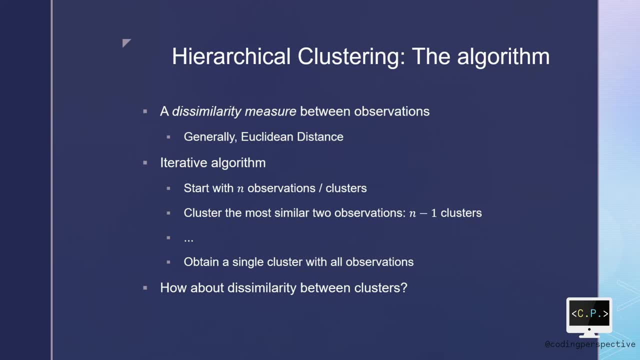 the clusters obtained by cutting the dendogram at a greater height. We will introduce the hierarchical clustering algorithm. We start with defining a dissimilarity measure between each pair of observations. This is generally selected as an Euclidean distance. however, there are multiple of them. The algorithm proceeds iteratively. 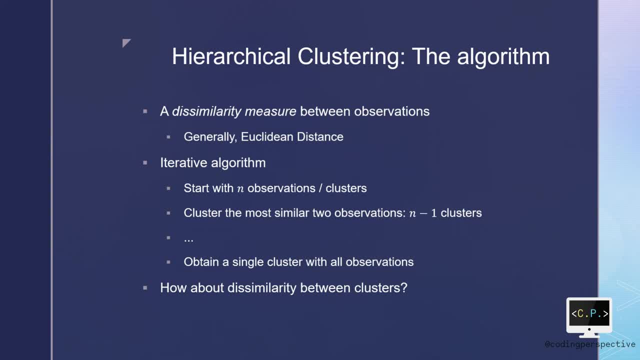 starting out at the bottom of the cluster and ending at the bottom of the cluster, At the bottom of the dendogram, each of the n observations is treated as its own cluster. The two clusters that are most similar to each other are then fused so that there are now. 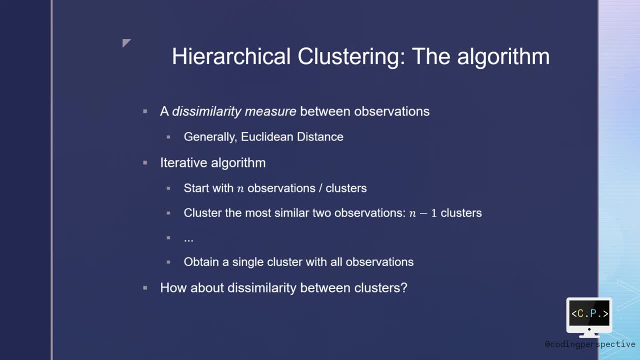 n-1 clusters. Next, the two clusters that are most similar to each other are fused again, so that there are now n-2 clusters. The algorithm proceeds in this fashion until all observations belong to one single cluster and the dendogram is complete. As you can see, the algorithm is pretty simple, but one thing is not. 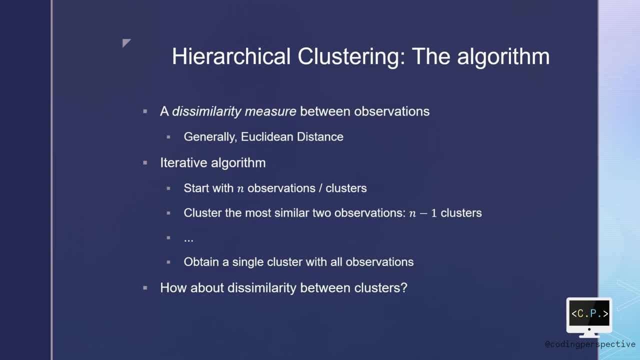 addressed. yet We defined a dissimilarity between pairs of observations, but we did not define the dissimilarity between two clusters. What happens if one or both of the clusters contains multiple observations? The concept of dissimilarity between a pair of observations needs to be extended to a 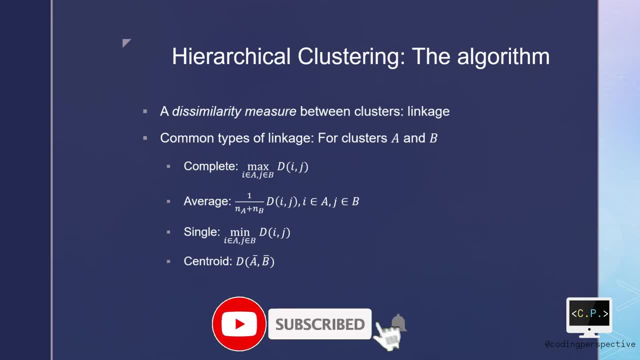 pair of groups or observations. This extension is achieved by developing the notion of linkage, which defines the dissimilarity between two groups of observations. The four most common types of linkage are: complete, average, single and centroid. In complete linkage, we define the distance between two clusters to be 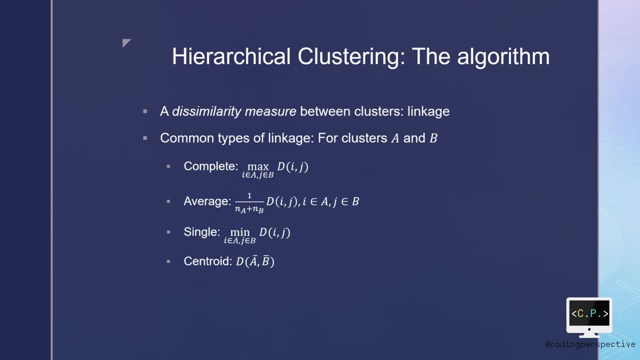 the maximum distance between any single data point in the first cluster and any single data point in the second cluster. Based on this definition of distance between clusters, at each stage of the process we combine the two clusters that have the smallest complete linkage In average linkage. we define the distance between two clusters. 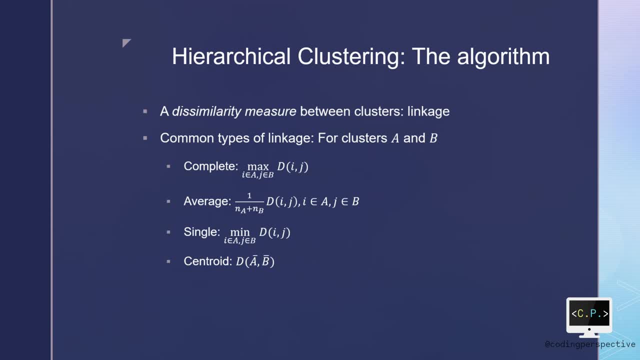 be the average distance between data points in the first cluster and the data points in the second cluster. So at each stage of the process we combine the two clusters that have the smallest average linkage in distance In single linkage. we define the distance between two clusters as the 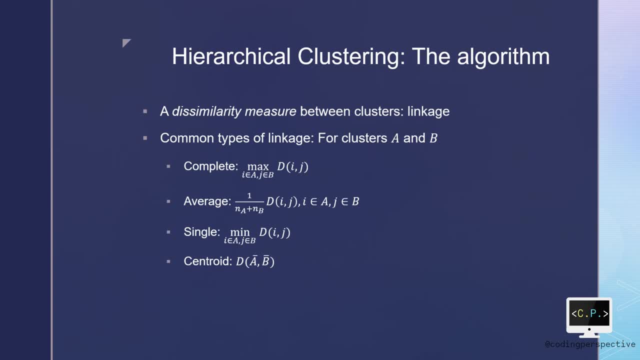 minimum distance between any single data points of the clusters. Thus, at each stage of the process, we combine the two clusters with the smallest single linkage distance. And last, in centroid linkage, the distance between two clusters is the distance between the two mean vectors of the 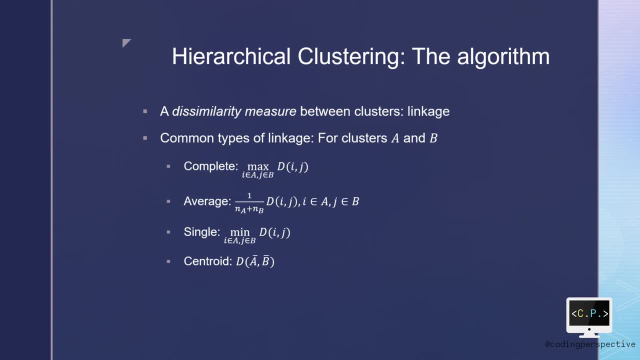 clusters. So at each stage of the process we combine two clusters that have the smallest centroid linkage in distance. So in our algorithm we begin with n observations and a measure such as Euclidean distance of all pairwise dissimilarities. We treat each observation. 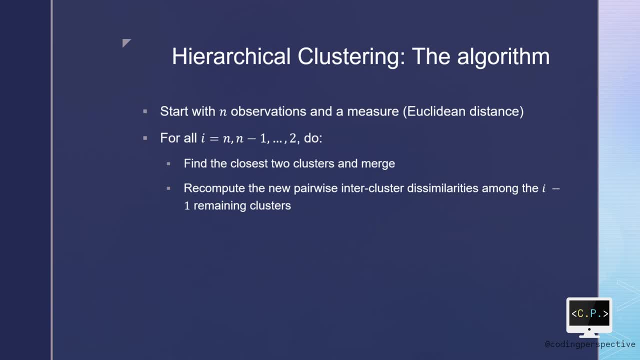 as its own cluster. For i, starting from n till 2,, we do the following: Examine all pairwise intercluster dissimilarities. among the i clusters, We do the following: Examine all pairwise interclusters, Then identify the pair of clusters that are the least dissimilar, which is the most. 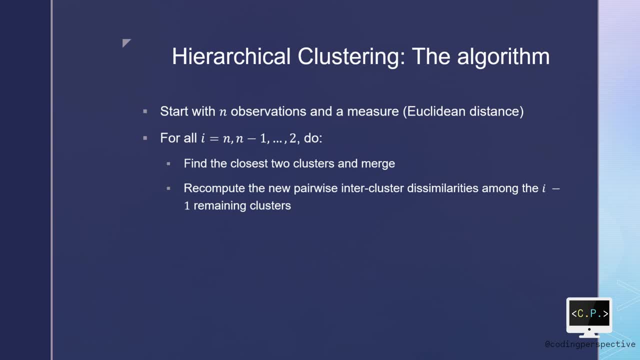 similar ones, Then we are going to fuse these two clusters. The dissimilarity between these two clusters indicates the height in the dendrogram at which the fusion should be placed. Lastly, we compute the new pairwise intercluster dissimilarities among the i-1 remaining. 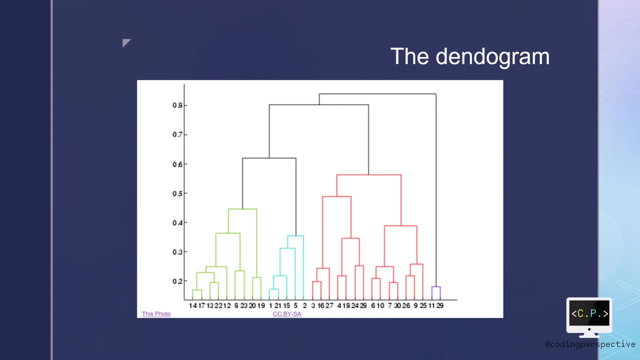 clusters. Let us have a look at the dendrogram, which is a result of a hierarchical clustering algorithm. I took this dendrogram from an internet source. Each leaf on the dendrogram represents one of the observations in our dataset. However, as we move up the tree, some leaves begin. 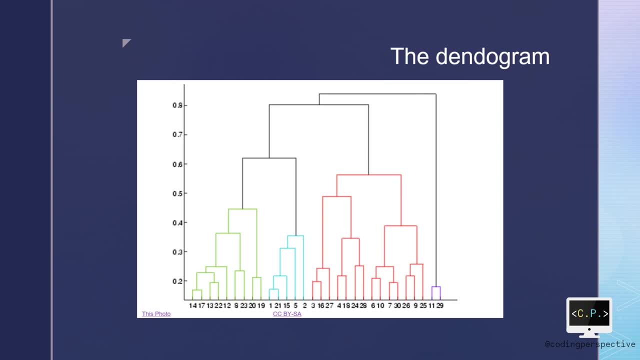 to fuse into branches. These correspond to observations that are similar to each other. As we move higher up, the tree branches themselves fuse either with leaves or other branches. The earlier fusions occur, the more similar groups of observations are each to other. 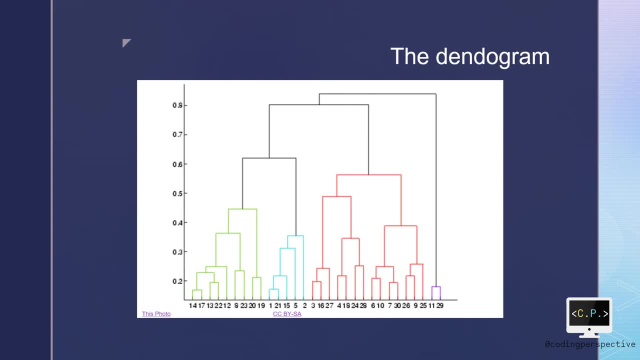 On the other hand, observations that fuse later can be quite different. In fact, this statement can be made more precise For any two observations. we can look for the point in the tree where the point of observation is the point of fusion, For example, we can: 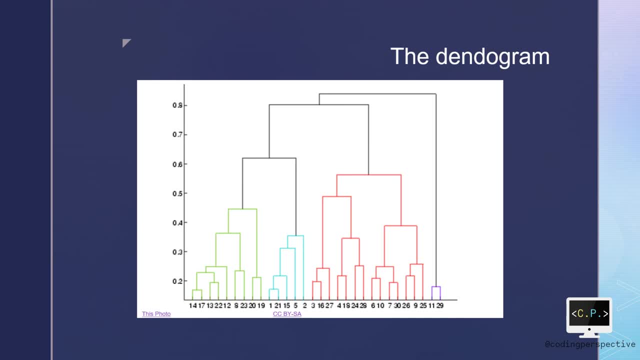 where branches containing those two observations are first fused. The height of this fusion, as measured on the vertical axis, indicates how different the two observations are. Thus, observations that fuse at the very bottom of the tree are quite similar to each other, whereas observations that fuse close to the top of the tree will tend to be quite different. 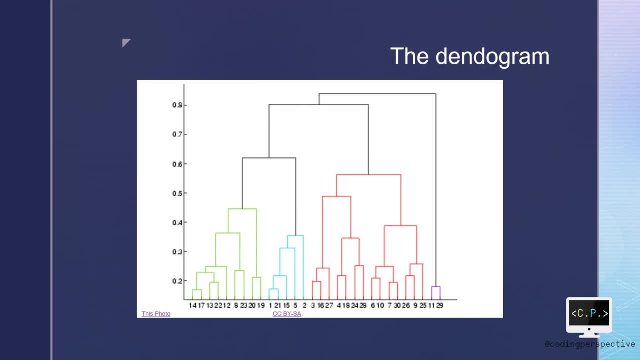 from each other. Therefore, we cannot draw conclusions about the similarity of two observations based on their proximity along the horizontal axis. Rather, we draw conclusions about the similarity of two observations based on the location on the vertical axis where branches containing those two observations first are fused.